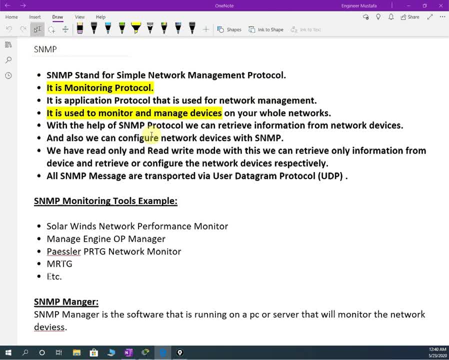 Some of our subscriber is also asking how we are going to monitor our network and how we can do. See, actually we have in our syllabus also, So let me read where we have this one. If you see our syllabus paper, that is PDF or any paper whatever we have in our Cisco site. 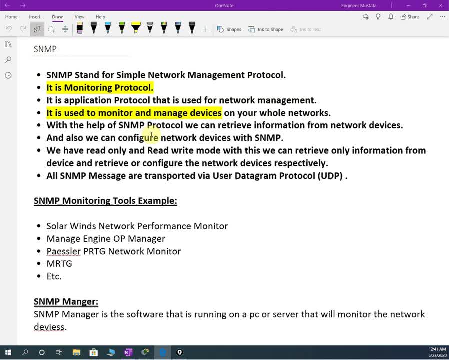 If you see 4.4, we have explained the function of SNMP in the network operation. We don't have configuration troubleshooting verification. We don't have. Only we need to explain the function, how it is working: SNMP in the network operation. So we don't have more. 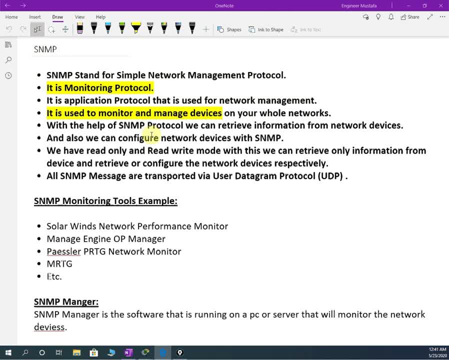 detail. here In CCNP we have a little more detail, So anyhow, let's start. You will be thinking why we want to use this. What is this? Okay, So before going, let me tell you if you have in your organization. 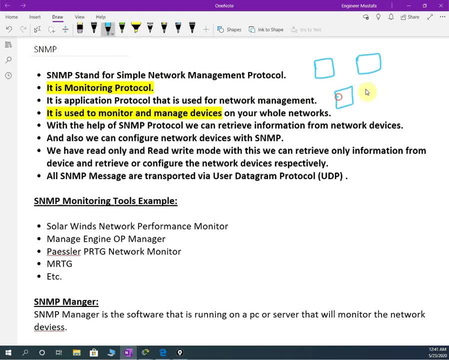 three switches or four switches and two routers. no need to worry, You can monitor daily, You can log into the switch or you can SSH or you can Telnet. sitting from one PC, From your laptop, you can SSH or Telnet the switches. 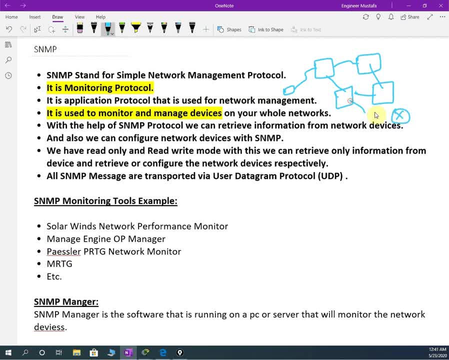 Apart from the narratives and router, whatever you have in your organization- And you can check the status: everything is okay or not, Or what is the issue, or like this. But imagine if you have, like, a network where you have more than 300 switches. 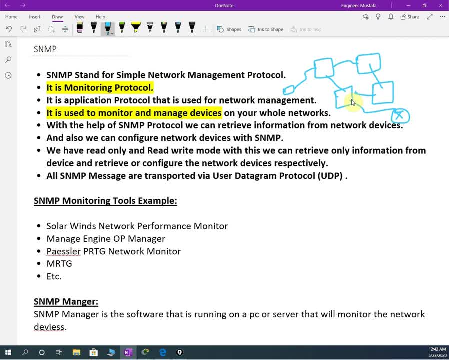 15 to 20 routers and dozens of servers and PCs like laptops. It is very difficult to monitor, right? It is very difficult if you want to monitor a big network in a big space. Right, It is very difficult if you want to monitor a big network in a big space. 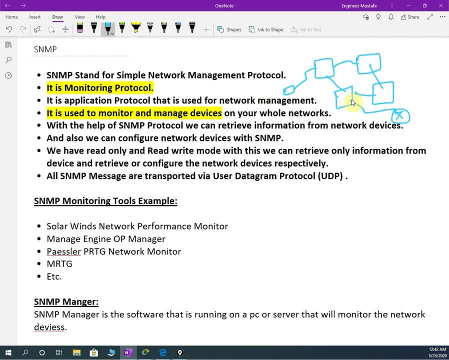 Right, Okay, uff. big organization where we have more than more than 100 or 200 switches, more servers, routers- all you need to monitor. if you are login individually, it will take long time and it is very difficult to look like that way also. so, how you can do what you will do, how to overcome. 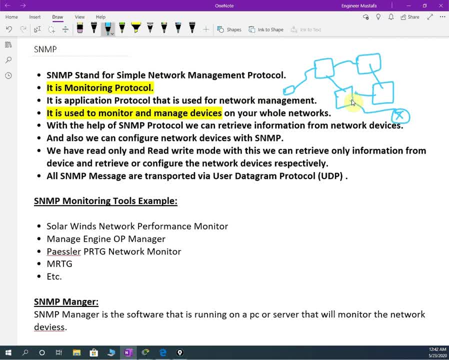 these types of issue. you will use snmp protocol to monitor the network devices. snmp stands for simple network management protocol and this is very important protocol and you can say this is a open standard protocol. snmp is an open standard for networking. network monitoring means you can. 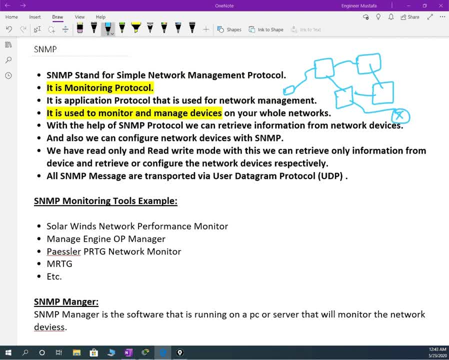 run this in any vendor, not only cisco. any vendor, and we have two types in this. one that is snmp manager as well as agent. manager is nothing but a: take one pc and install the application that we can say as a manager and the agent is our networking device, whatever device we have. 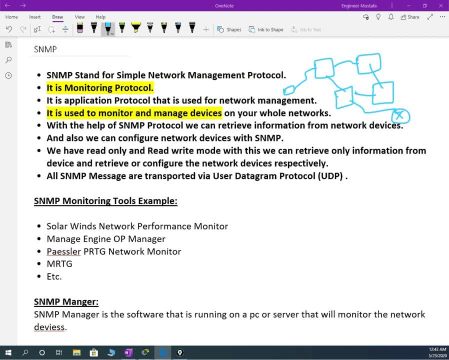 like ip base. we can say that is the agent. but anyhow, let me revise here, let me go point by point. so first of all, this is a full form. we know and in simple words we can say it is a monitoring protocol. it is a application protocol that use for network management and it is used for monitoring. 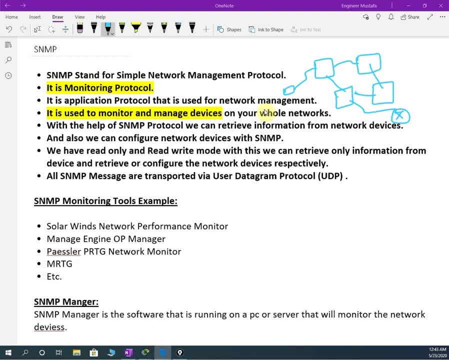 the network, monitoring and managing the devices on your network. so with this protocol, you are not only going to monitor, you are going to configure also. you can monitor as well as, if you want, you can configure also. with the help of a mp protocol, we can retrieve the information from the network. 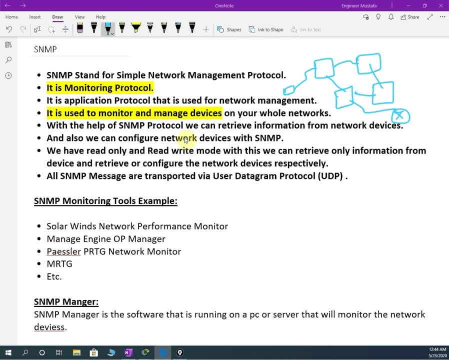 device. and also we can configure the information from the network device. we have read only or write only mode. with the help of that mode, whatever we consider is operating the device configure, we can do reading, we can do reading operation or we can do writing operation. okay, all snmp messages are transmitted via udp protocol, that is, user datagram protocol. we are 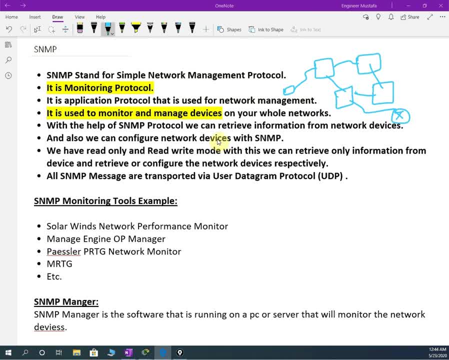 going to discuss some basic. we did not discuss what is udp because everyone know tcp, udp. that's why i did not cover, but anyhow, make a list. whatever we did not cover, we are going to cover that one, okay, uh, if some of the guys who is working in an organization, if you are working in 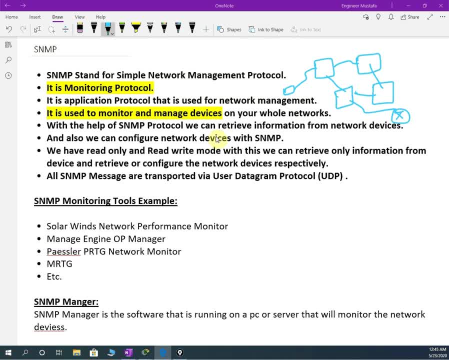 telecom or anywhere. you will understand what is snmp. remember a long time, or now. also, everyone is saying i am a knock engineer, network operation center. he is sitting in the knock and he is monitoring the network. same that is also snmp. he's checking if any alarm is coming from site. 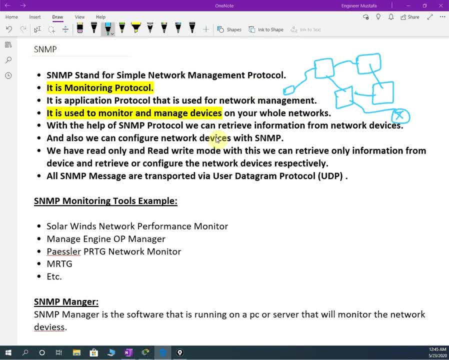 he's calling the team and he's saying to the team: there is alarm, go to that site. same thing: if you are working in a telecom or anywhere, you will understand what is snmp. same here, also in networking devices. we are using one software, that is snmp. we have different. 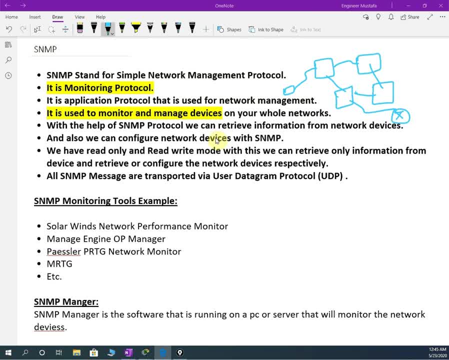 vendors of software. we can install, we can buy some free source, also available, open standard. that is like we have free tools also you you want to use, you can use. you can install in your machine to check that one and we have paid one. also in organization we are taking the paid one because 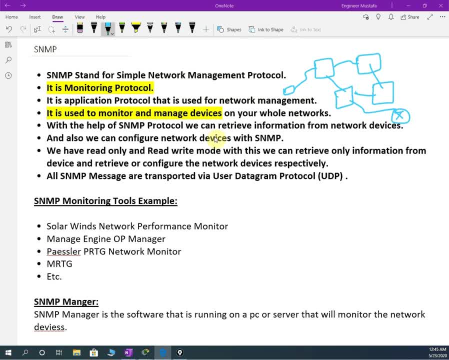 we need trust and everything license one. we don't want to do that, so we are using one of those to use any uh, like any open voice, open one without license. so we are using the license one in our organization. example, we have solar wind uh network performance monitoring tool. this is one. 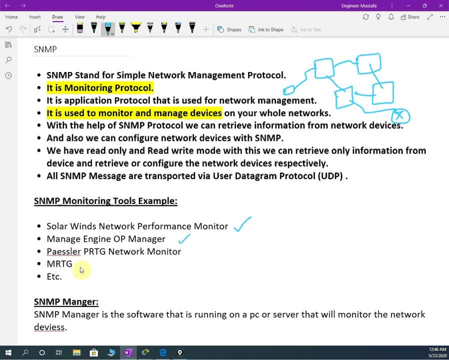 manage engine op manager and this one, mrtvg. you can try to look in google. this is a software we can install in our pc. in simple words, we will say: snmp is a monitoring tool. it is used to monitor network, like if, as i told you example, if we have 300 devices and you have the 15 router in your 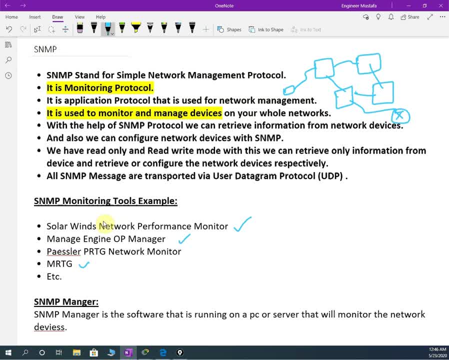 organization and many pcs it is difficult to monitor like you can configure in this one. if this router is using more cpu or more ram, or if it is a interface, go down. please send me message or notify. it is a application you install and monitor the network like this protocol, collect the data. 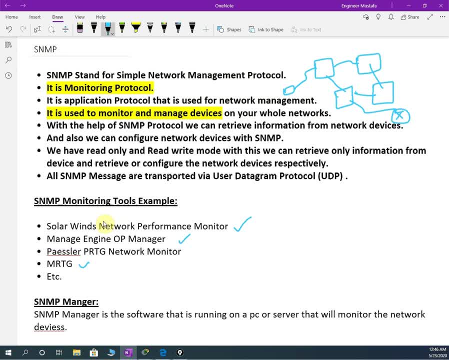 from the uh networking device. he will send some request to get the information and it will plot in the graph. you can see in the graph what is happening from last week, one week, one hour before and one year before. like this you can see in simple words. we can say it is a monitoring tool. 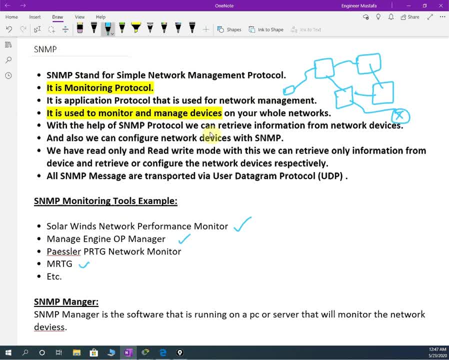 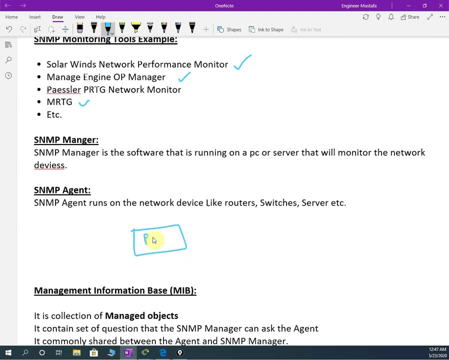 okay, with the help of snmp protocol, we can retrieve the information from network devices, as we discussed already, and this one already we discussed, and this is example. let me tell you what is manager and what is this one example i will see. this is a one pc, okay. 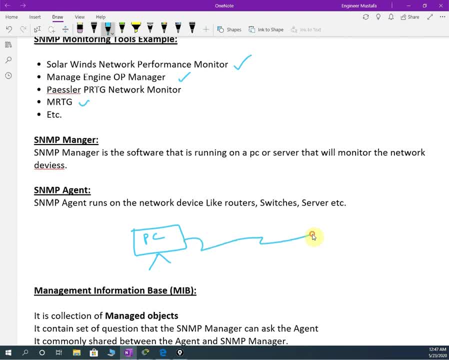 i am saying this is a one pc, this is computer. it is connected to router. i am taking- this is a simple example: in one router you will have two router or fifteen router of to like hundred switches like this here. this is a big topology but our simplicity, i am. 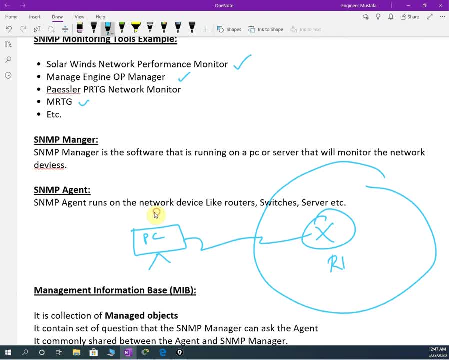 taking one pc and one router. so this one you can say sn, mpa a manager, we install the application here, so that application is running here. and we can say snmp as a agent, so router or whatever network device. not only router, we can have printer, uh pcs as well as. 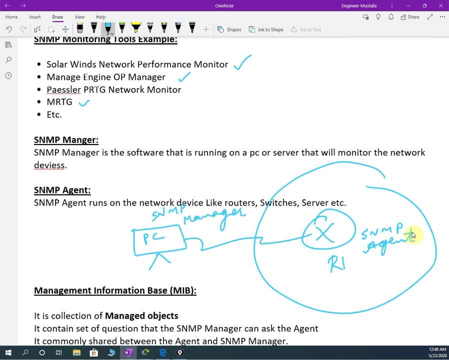 switches, i all ip base thing. whatever we have we can configure. so if anything go wrong we can get the message or email, depending upon the configuration. what you configure and also you will get in this pc. so in this pc you can observe what is happening in your network. 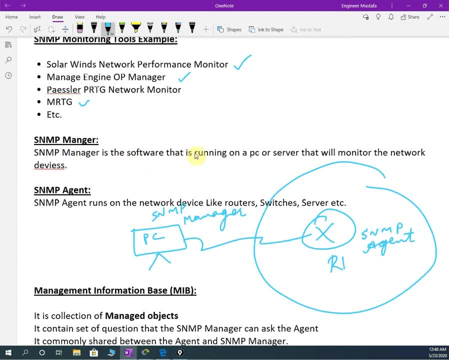 so sns nmp manager is a software that is running on a pc or a server that will monitor the network device. okay, and sms nmp agent that is run on the network device like router, switch or server. okay, i hope you understand right. this is simply simple topic. we have only theory, we don't have. 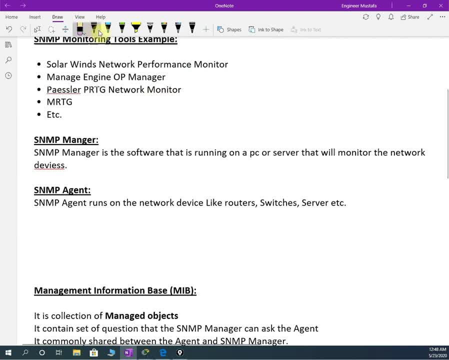 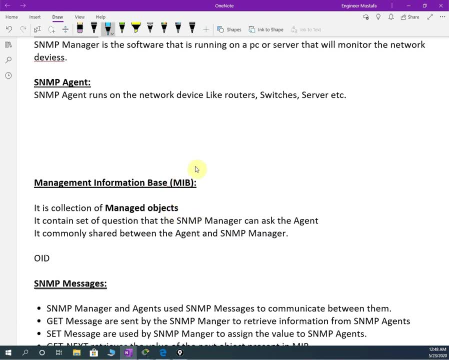 configuration. but we are going to do configuration. we will try to do configuration also in our lab. okay, you in this one. we have a management information base. we have one database that is management information base. it it is collection of managed object means. in this database we have information. 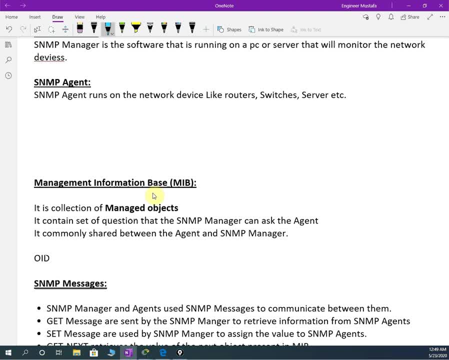 whatever we need to pull from the devices, depending upon the different vendor, they have different uh features. whatever we need to like, every one minute we need to check the status of router, check the interface status, check the temperature of the router and check how many how much ram is utilizing. what is the cpu, how much cpu is utilized and what about the switch. 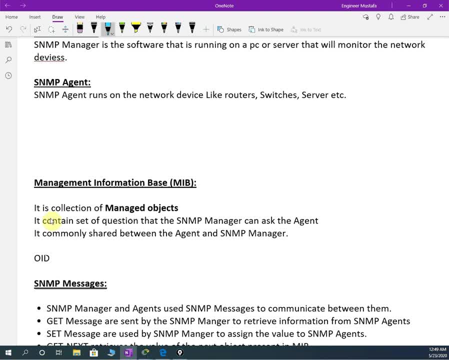 we have so many things that is present in mib so we can say it is a collection of managed object. it contains set of questions that snmp manager can ask with the agent and it is commonly shared between agent and manager. so this is a one. imagine this is one database. whatever question, 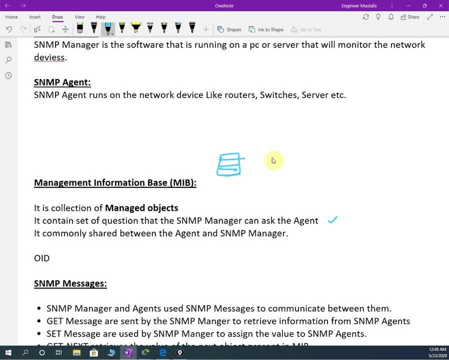 we need to ask with them, with the router or switch or whatever networking device, that question all is written here and this is shared between the manager. this is a manager and this is a agent. we will share between them. so every one second, depending upon the time, whatever. 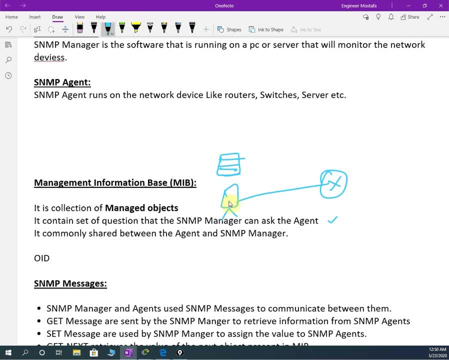 we keep like one minute or two minute every that time time period. he will send the request and they will send the status and it will plot in the graph. it will show you what is going on here. so we have messages. what messages we have, let's discuss snmp. manager and agent. 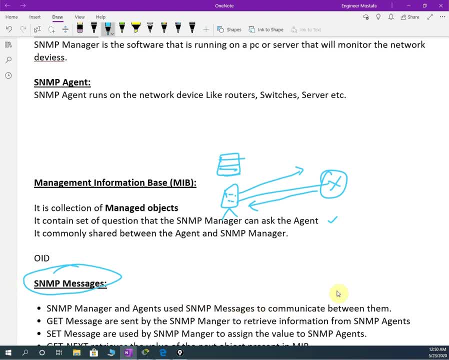 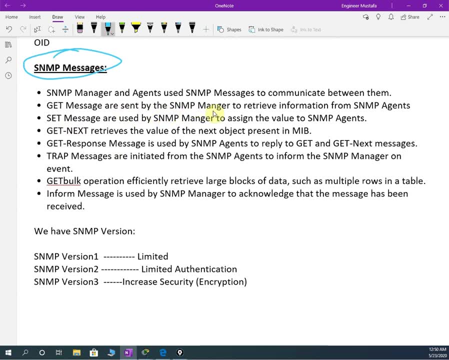 use snmp messages to communicate between them. okay, and what messages they are using. they are using get message are sent by the manager. manager is going to send the message. get to retrieve the information from the agent. and set message are used by the manager to set the information. means if we want to configure anything, we will use set message to set the. 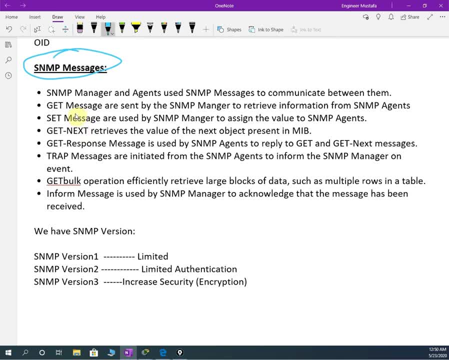 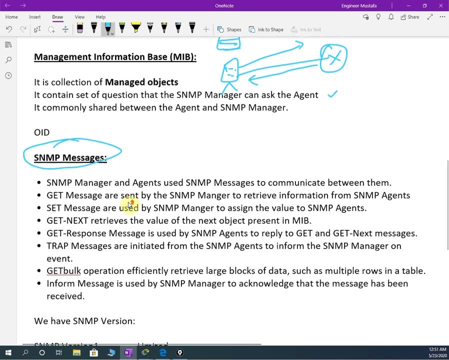 make the changes in the configuration, but we are getting information. then we will write get message and get next retrieve the value of the next object present in the mib. okay, what is mib? we already discuss here management information database. so this is a database, management information base. we can say this is a simple database which is having whatever. 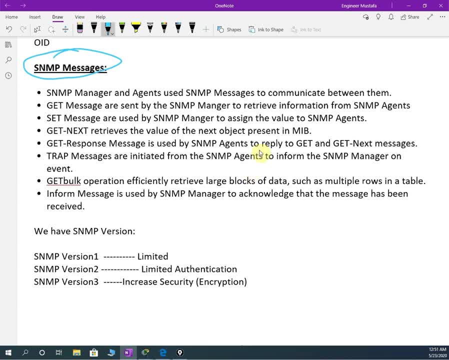 question we are going to ask with the agents. okay, and get response. message is used by agent to reply to the. what is the agent? okay, and get message is used by agent to reply to the to get message. so, with this, get response. they are going to reply whatever status is there and 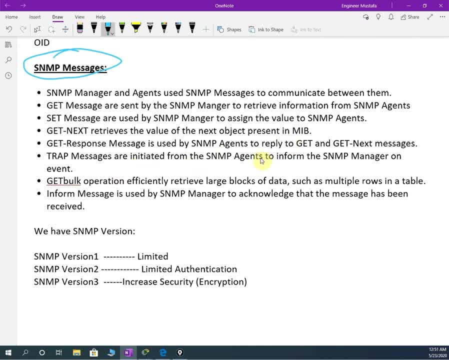 trap message also initiated by the agent, like if this is a router and this is a our manager, every time manager is sending something, they are replying something, but suddenly something happened wrong without asking him. they can send them without, like. this guy is asking what is the. 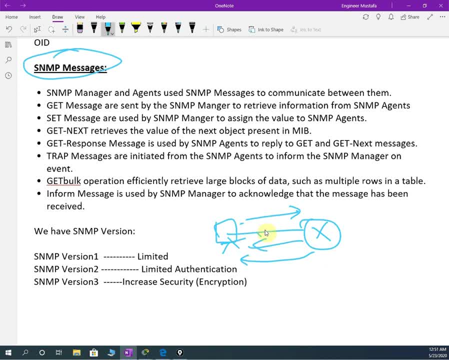 status of this question. he will reply, but within the duration or before asking this one or if any other event happened, it is configured, then he can send that. he also like he will say the interface of this one is done. it is not present in your question, but i am saving that information that. 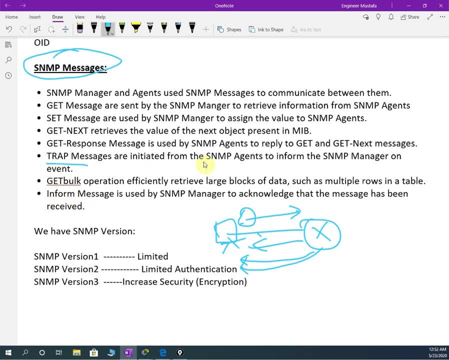 information we will get with the trap message. trap message are initiated by the agent to inform the manager on the event. any event is that is happened. he can, you can get the message and then he will reply, but within the duration or before asking this, one himself also can tell that this is a problem we have by the trap message. okay, and get, get bulk. 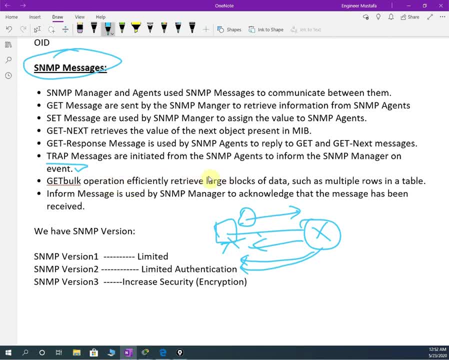 message is also there. we can get the large data, not sending one by one. we can get more data and this is a informed message is used by the manager to acknowledge that i receive the data. and in this one we have three protocol, that is, snmp version one, version two and the then version three. and 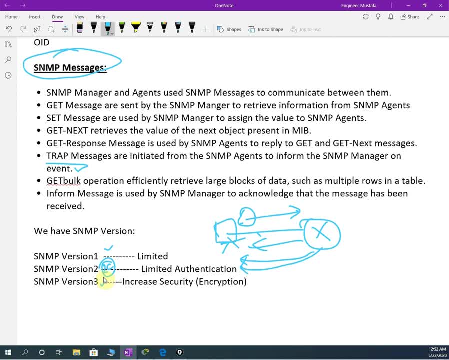 version two. we have to see we are saying we will discuss that one also. so version one, version two, version 3: we have here limited, that is, limited feature we have here. we have more feature but limited zodication in this we budget. and 3, we have more security, that is. 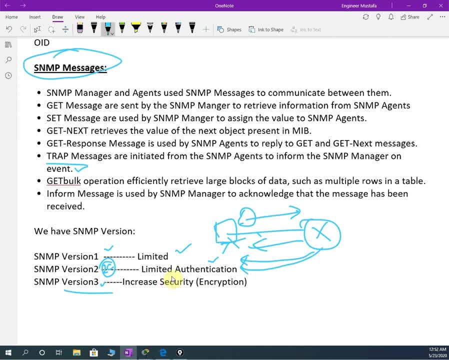 encryption as well as authentication. we have. so what we are saying, let me breathe one more time. ok, then we will see. if we want we can do lap. but actually in our syllabus we don't have lap. ok, so let me revise a cell. SNMP is a open state. if, let me revise, i have all the games, that is 992 really. so let me revise, lets have, this is what we have. ok, so what we are saying? his number of style, una one, is only no, because it is accessible only if i say by himself: this is, uh, my name, my name n Под to. we are working with a company that is aagt the same one. e acept the date of when a body is changing is a row, and 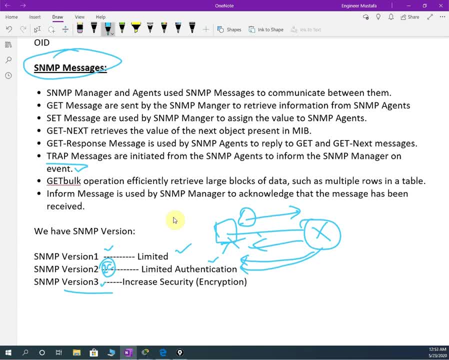 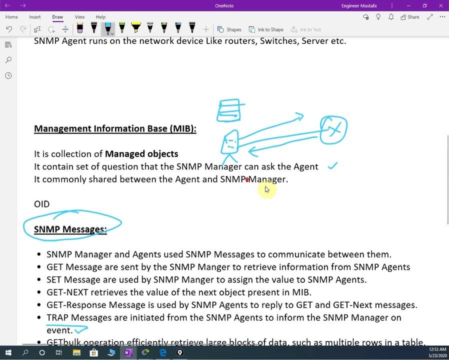 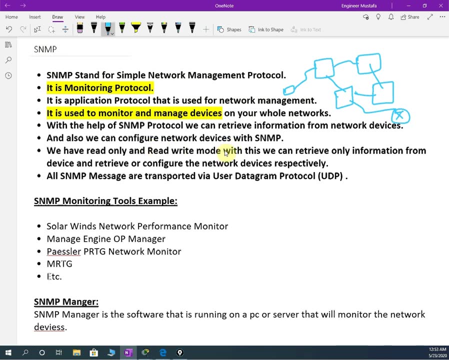 standard for network monitoring and it is having server as well as the client. server is used to collect the data from the client. what is client means? this is agent, who is going to reply that one, okay, and this is going to collect all the data and store in his memory and he will give. 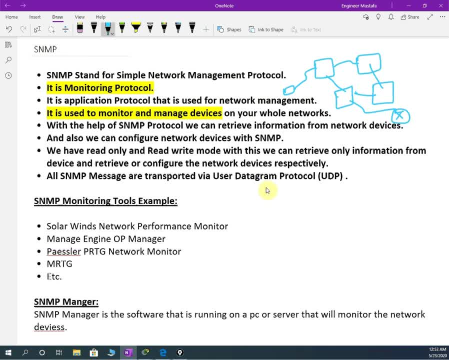 the graph and the what we can say, all the dashboard. in the dashboard we will have what is going on, what is the behavior and all that one okay, and data where, depending upon the SNMP manager system, are organized in the MIB. what is MIB? as we discuss, MIB is used because MIB is. 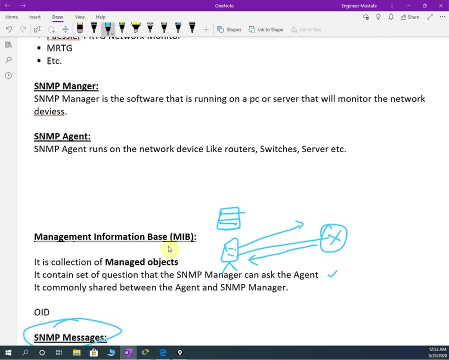 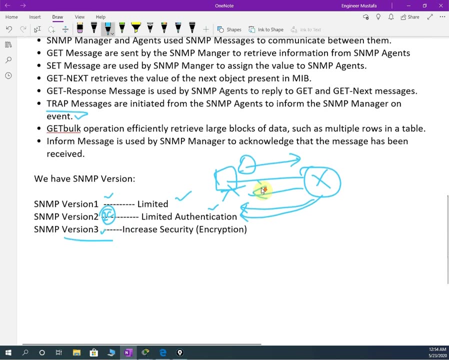 nothing but a management information base. it is having the list whatever need to check and we agent and the manager- both are share this question. they will ask and they will reply that one and in simple words we can say they are three types of version: version one, version two, version three. also in version one we have like 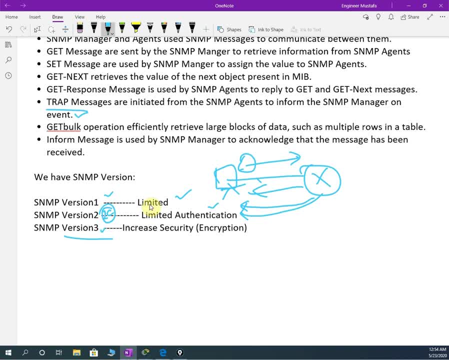 use plain text for authentication between the manager and agent and we cannot take the bulk information. but here in the version two we have like bulk information we can ask and in third one we have the support is strong authentication and encryption. it is prefer version but it is. 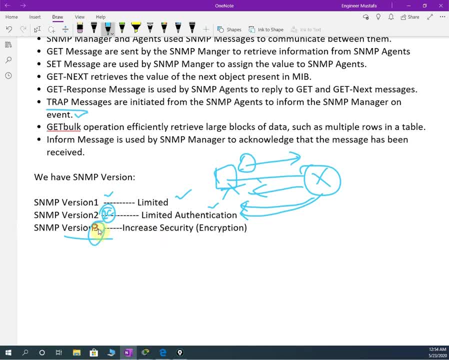 not supporting for all the devices for the version three, so mostly we are using version two or version three, depending upon the devices. whatever we have in our organization, okay, and we have a string also, like a string is nothing but a password we will have when we are configuring. we will write our RO that is read only, or RW to write only. this is a. 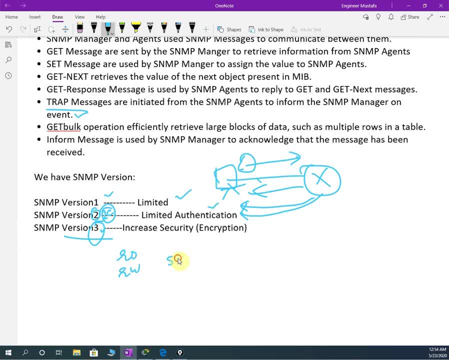 two types of string we are going to use, like SNMP, version 2c. we are saying: to see this one, we have advanced version, little advanced compared to version 2. we- we are saying 2c, use community community string rather than the username password. in this one we are not using username password. we. 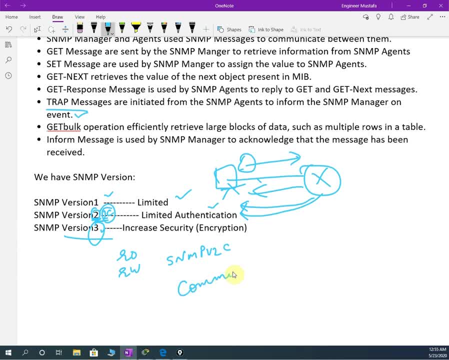 are saying community. let me write here community string. we are saying community string for the username and password. we are writing that community string. we are using community string rather than the username and password for the authentication of the SNMP manager and the agent. so whenever we are going to configure manager and agent, we are going to 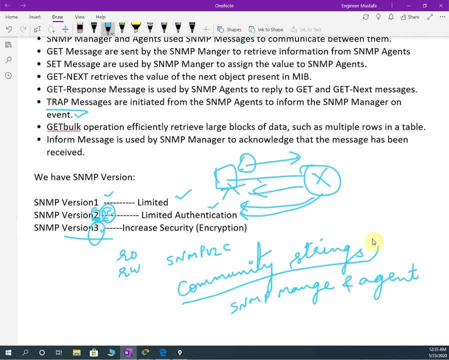 use the username password. but in here, in this one, we are saying community string, we are not saying username and password. I will show you what that one. so if match is found between the manager and the agent, then they can communicate and we can write. read: only community is used for manager. 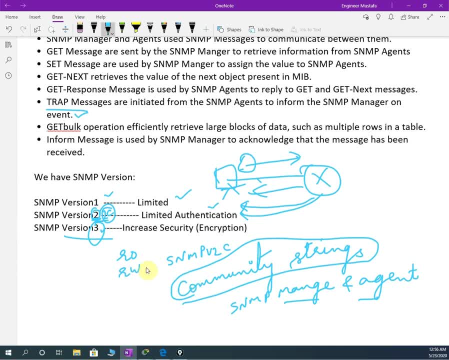 to read information and write only string we use to use in the manager to have the permission to read as well as write the configuration or set the configuration. if you want to make some changes in the configuration, we can do that one also, okay, so let me erase this one. 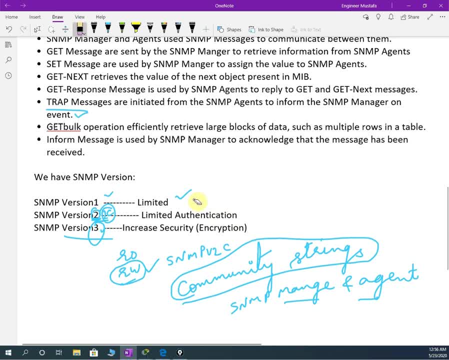 and then I will write some commands and let me show you also in a basic packet tracer, actually what we will do. we will install one application in our client PC and we are going to configure the SNMP protocol in our router or switch. and then we are going to do: but we don't. 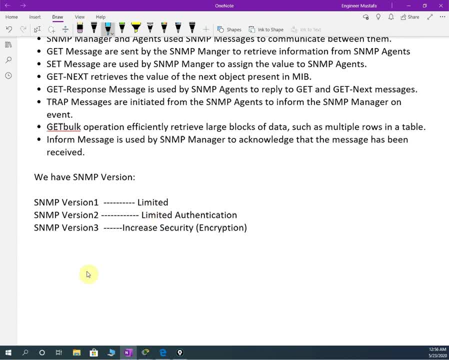 have the lab in our what we call in our CCNS labels. but anyhow, example: see, this is a router R1 in the configuration we have in the configuration mode. so we need to write. we have like this, so what steps we will write? we will write SNMP, space server, and here we need to write community. 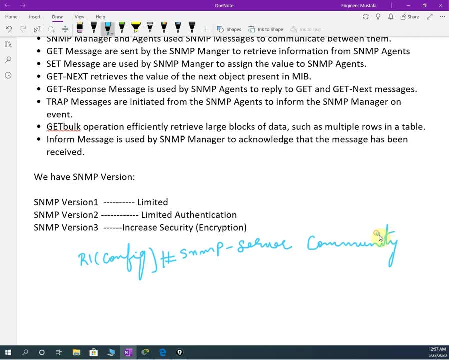 community and then you, whatever password or username you want to give, you can write: here, I will give ABC, and you can write RO. RO means read only same thing, we will copy from here to your community and here, if you want to give different name, you can give ABC one. and if 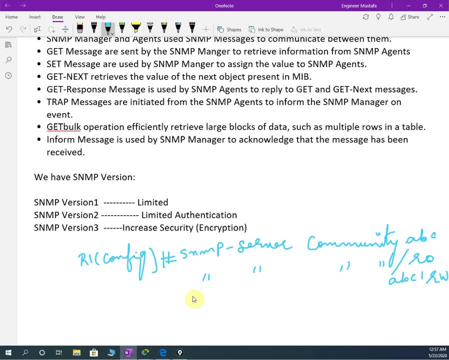 you want to give right permission, you will write right. so this is a configuration. after that, uh, what you will do, you need to define which one is the server. like you write SMMT server. I will do no problem, you will be confused. no problem. host. then you will give the host name. 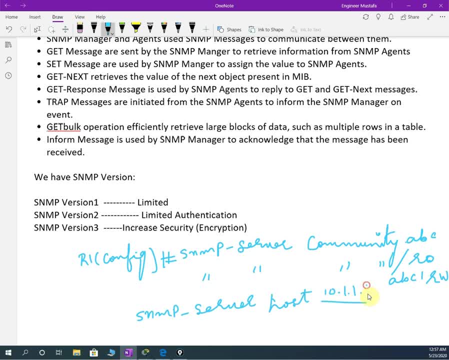 host name, that is IP address. whatever IP you want to give, 10 dot, 10 dot or something- then you will write the whatever permission you want to give, you will assign that one. okay, so anyhow, let me give show you there in the packet tracer. I will open the packet tracer here. see, this is the packet. 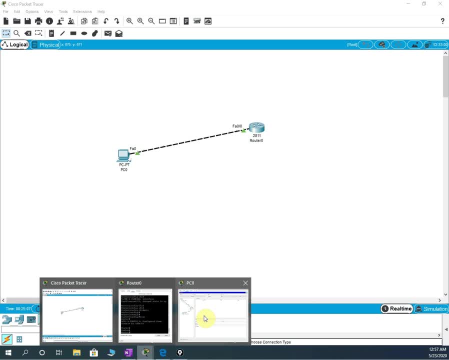 tracer. I already taken this one and let me close this one. so you will have the idea. but don't worry, you don't. we don't have configuration, troubleshooting, verification in our syllabus. only we have the theory: what is a tool and why, why we use this one, what is that one? only 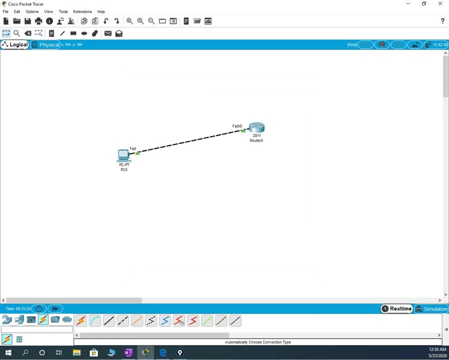 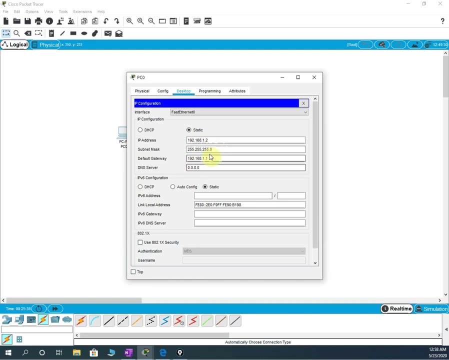 we have that one only. okay, if you want, I will show the configuration, no problem. so let me show the configuration. what we will do is this one. this is the PC we will take. I assign the IP address in the PC 192, 168, 1.2 and this is a default Gateway. uh, subnet mask and then default Gateway. I put the 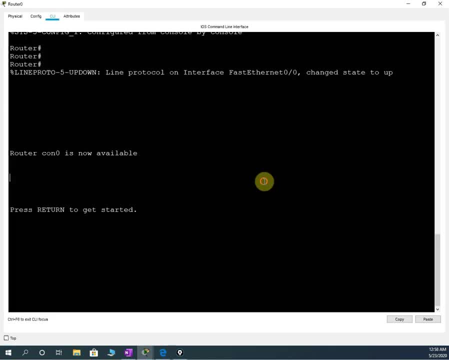 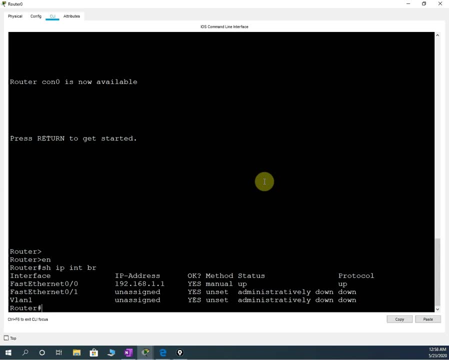 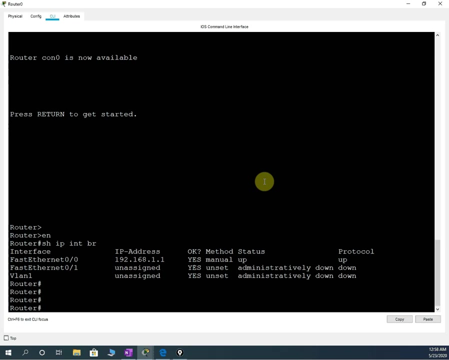 router interface. okay, and I configure the router and interface here. let me show you. if I write here, show IP interface brief, you will get the. I assign the one IP address here, okay, so now we are going to configure the SMT, SN, SN, MP protocol. okay, so if you? 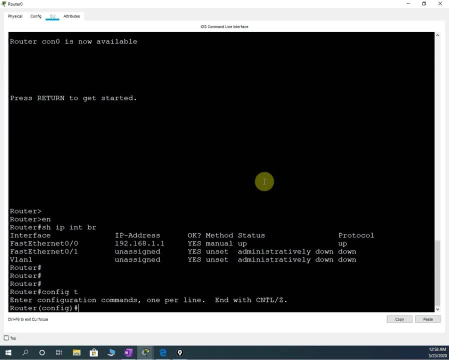 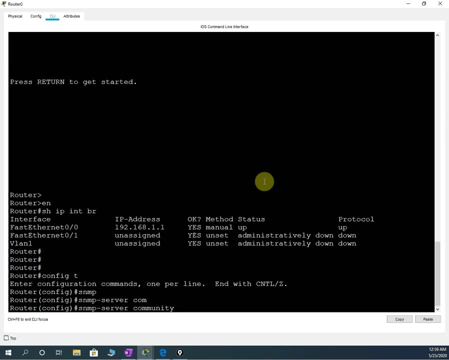 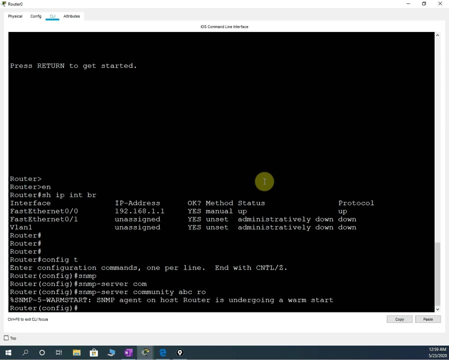 want to configure that one how we will give. we will go to global configuration mode. then maybe we write snmp server and then you can write Community and you, here you are writing the password. so I will write ABC. okay, ABC, read only so. ABC. password is only so here. snmp agent on the host router is undergoing a. let me see what is we are getting. 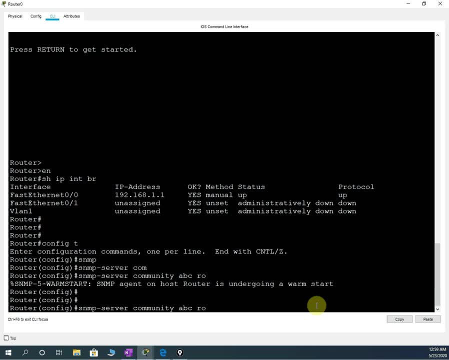 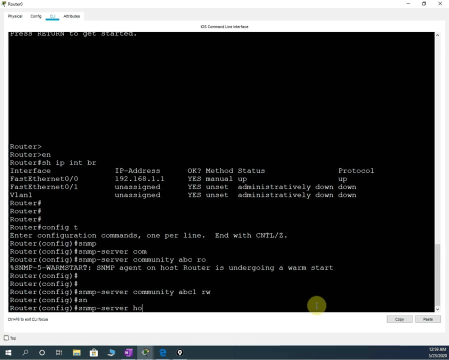 here warm start. it is saying so. anyhow, let's proceed and do that one. and here password: i will give abc1 and then i will write. i need to give permission for write also, so i will write, wr, write. so now what i will do. i need to assign the ip address for the host, so server ip address i. 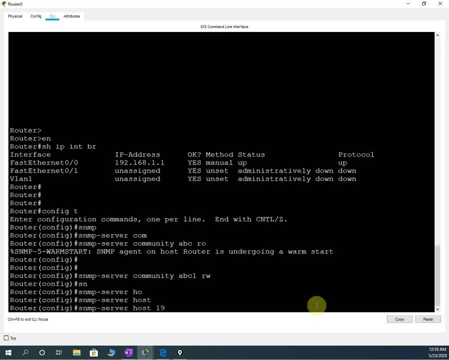 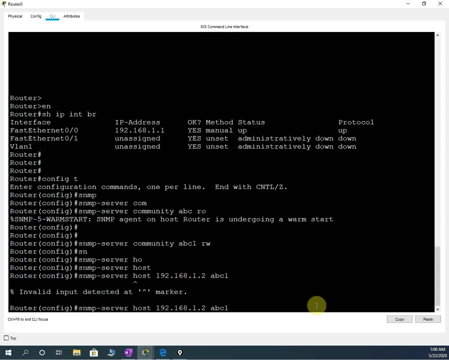 need to give. so what is ip address for the server? so server ip address: we give 192.168.1.2. okay, 1.2, and i will give abc string password. we need to give abc. i will give abc1. okay, so this one is not taking, so something we put wrong. let me check after this one, because i 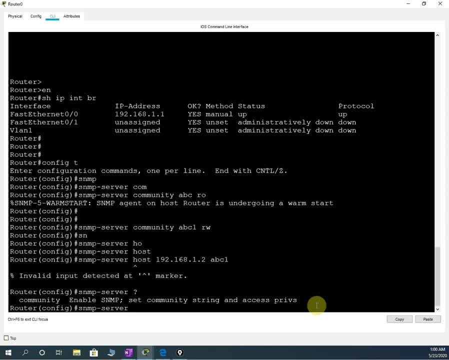 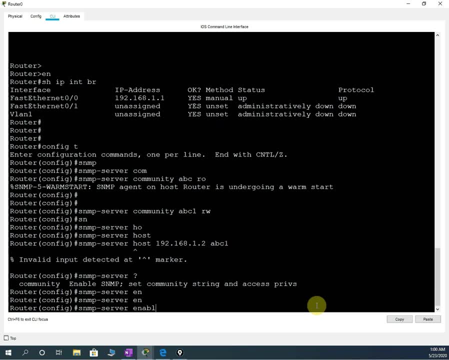 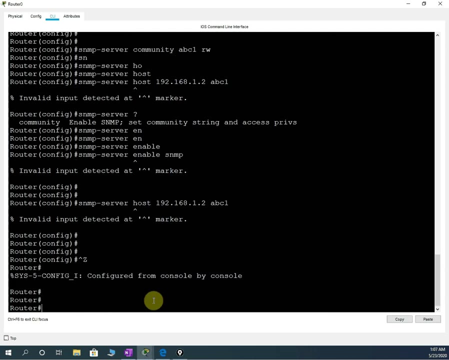 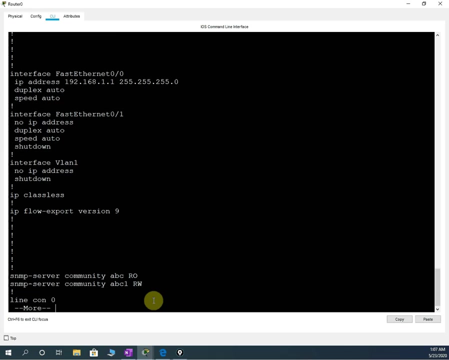 think packet tracer support or not. a server host is asking: write community, enable sms and empty. we need to write enable. let me write: enable this snmp. actually that command is not supporting in the packet tracer but anyhow, whatever we wrote, we will check show run. then we will see that one. let's see here. see so here. if you see we configure the snmp server. 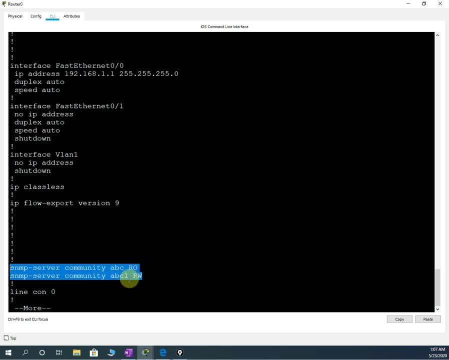 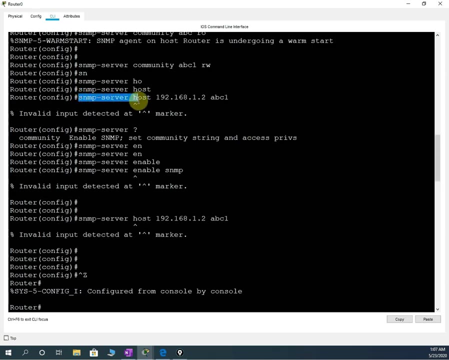 community: abc for ro and abc1 for rw. so now we configure this one. okay, but in real scenario we will see that one command, that the one which we are getting error in the packet tracer. if we do in the gns3 it will work, i hope, but here it will not accepting. we need to define the server. also what? 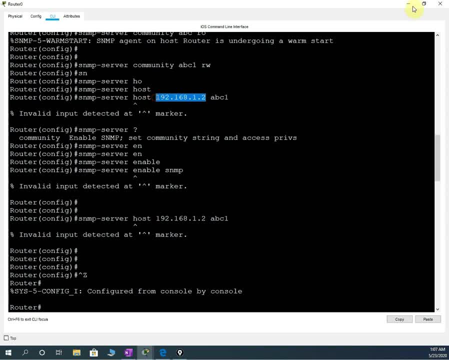 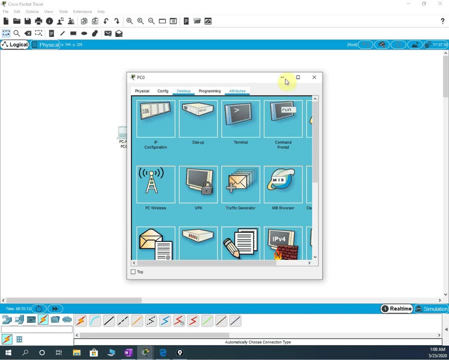 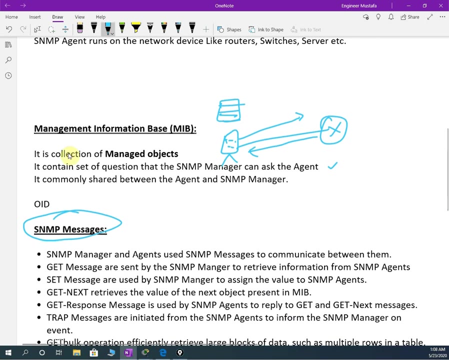 is the server. we are going to use that server. ip we need to assign, but as we are doing in packet tracer, so we will just enable that one. and then we will go here and in the pc we have mib. you remember mib? what is mib? if you see, here mib is nothing but a. and then we will go here and in the 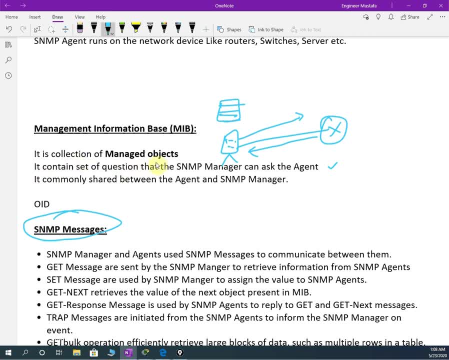 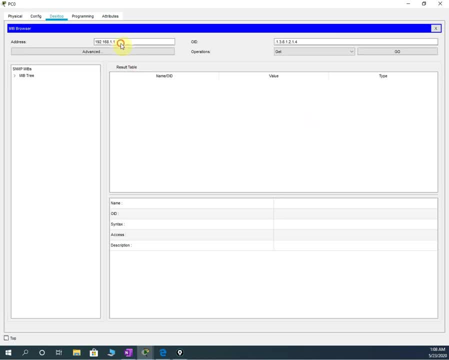 pc we have management information base. it is a collection of manage object. so in this we have the manage object. so when you purchase the software you will have this application separately. so i will write here the router ip address: 192, 168, 1.1 and advance. i will click. we need to add this first. 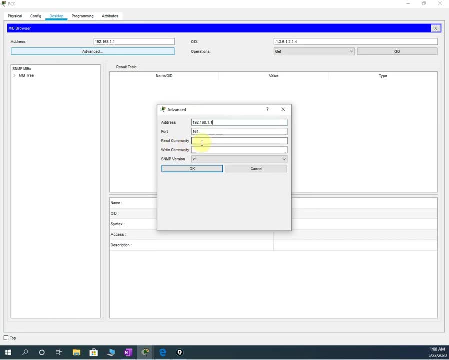 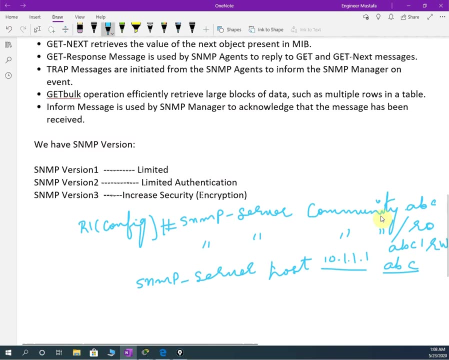 time we need to add. so this ip came: read string. what we give this is a password example. as i told you, here we don't have the username and password. we need to give only the read and write string. so for the read arrow only and read write is abc one. okay, you remember, in the router we give that. 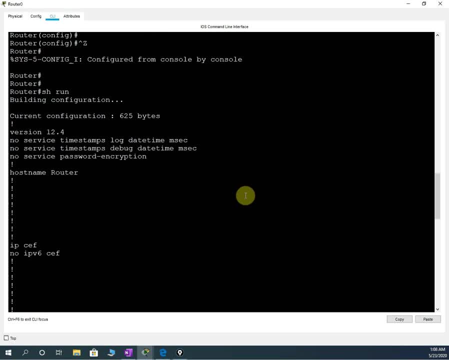 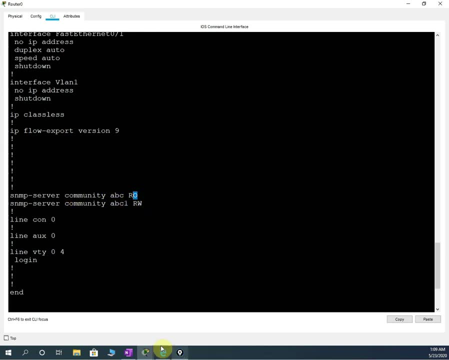 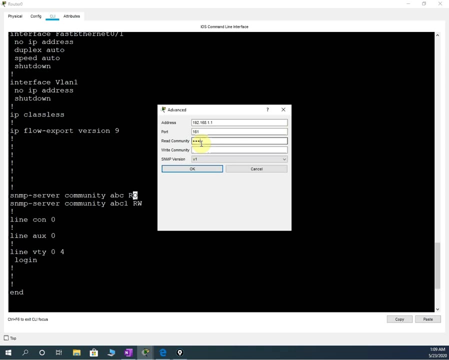 configuration, if you remember, let me show you. if we write show run we have here for read only we give abc for read, write we give abc one. so what i will do, i will go in this advanced setting, in the read only i will give abc, and here in this one i can give abc one. and here which version we want: 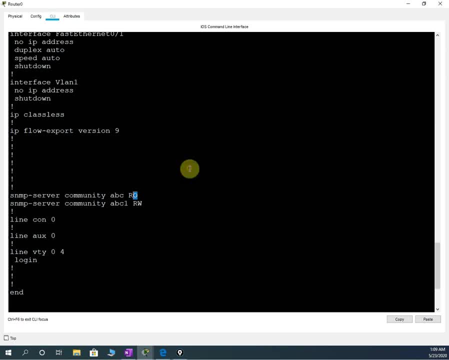 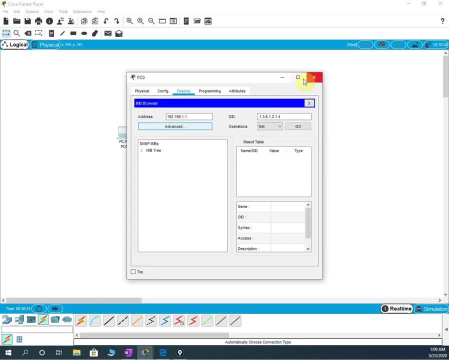 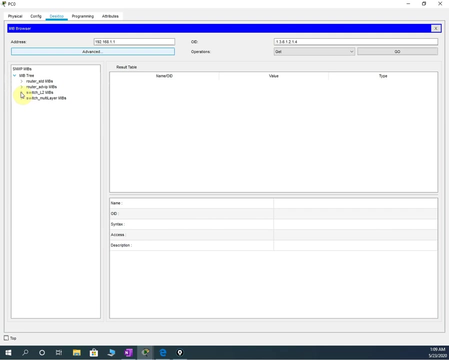 so nowadays we are using versions three, so i will click version three. okay, so i set this one. then let me go to the packet tracer. i set this one in this one and we, if we maximize this one, we can go in this tree. we have the router, we have the switch, whatever the vendor define, we have this all here. 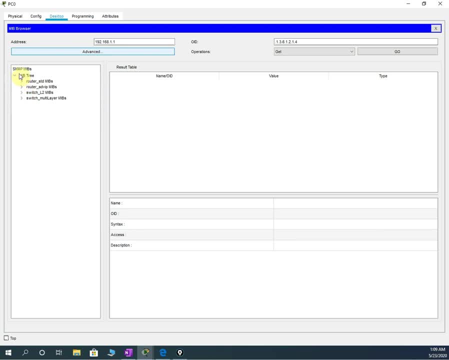 okay, so now what you need to do. whenever you purchase the license version, you will have like this: you have different parameters, so i will click this one. i will see what we have in this one. if you go arg and here interface, if you go here in this management. 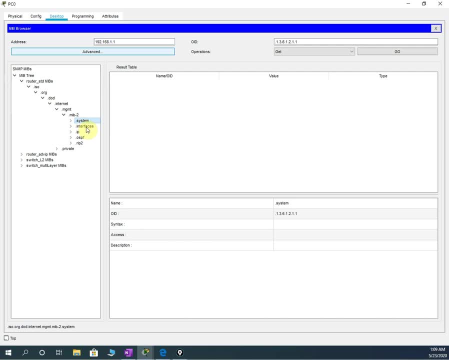 uh, if you see we have the system, and if i select the system and i will write uh, get here, i will write get and then i will click go. he's saying command error because we did not select the term. let me. oh, id. id is coming. this is okay. what issue we have? 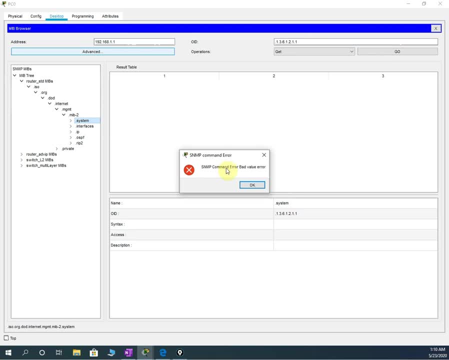 it is giving get we selected and we selected a bad value. it is already maybe this one. which router we have router. we have one router only. okay, so let me check which one actually we don't have in our syllabus. but anyhow, i am doing this. we will do in ccnp for gns3, not here, if you see here. 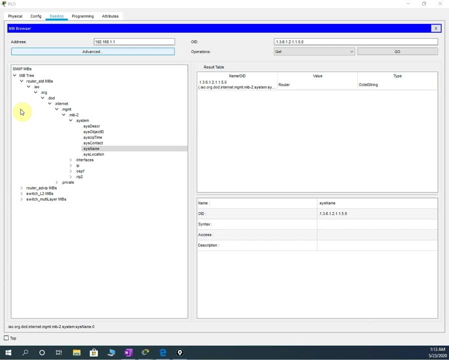 now we have. so let me tell you see, first of all, what we will do. we have, uh, first of all we need to add the interface of the router which we configure. okay, so I will put that IP address, I will click this connect. then it will ask the read Community, right, Community. so whatever password, we 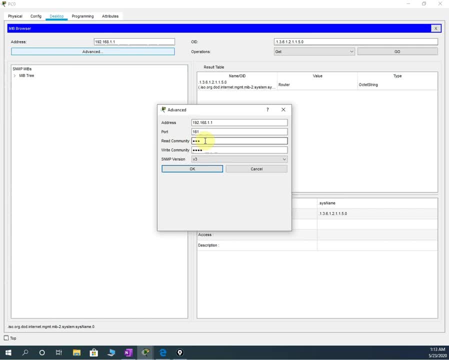 give. we need to write: I give ABC. I wrote ABC here. this is ABC one and which version we need to use. we need to write that one and press ok so it will interconnect. then press here and then we will have the first one. we will select this and then we will go inside and then in this tree, if we go system. 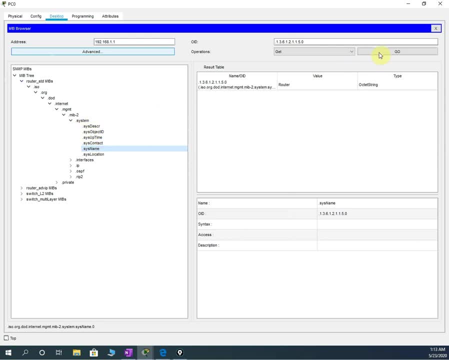 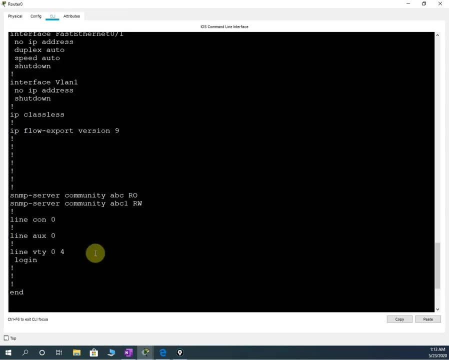 then we have system name. so if you select system name and press get, you will have the router, because our system name is the router here. if you see router, let me see show. this is the router. if I change the configuration here- host name like- I will write R1. okay, I will write R1. we have R1 now. 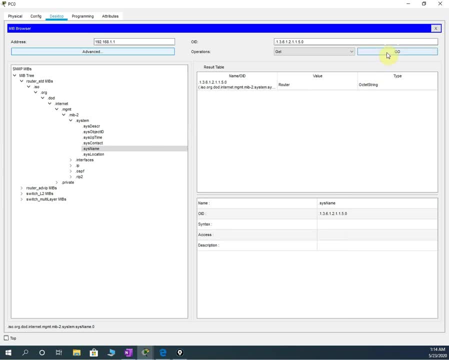 so now let me again put get see now change to R1 before we have R, and if you want to see some more see sub time or anything, you can select and you will get. whatever time and object, depending upon different vendor software, we have different feature. if you want to see the interface or 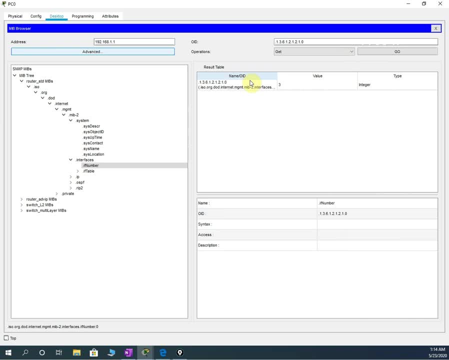 in interface, what is like values, and depending upon the manufacturer, we have different feature. this one, so name, we can check, and the description, like here, what we have, the software, we can check. that one, okay, let me show you the. this is a get command we use. okay, if I want to write set, I can write set command. 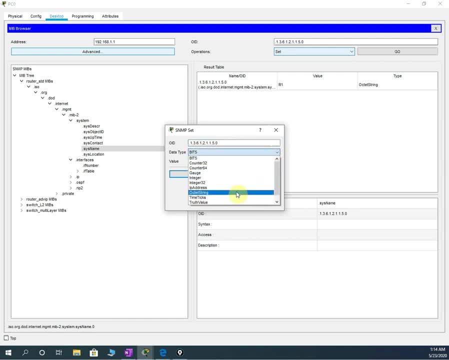 also in the set command we will use the, this string and what value you need to set. so example: I want to set R2. okay, so I will write R2 and then I will press this one and then I will say: go. so now I set the R2. okay, if you go in the router and you will check, it will change the settings. 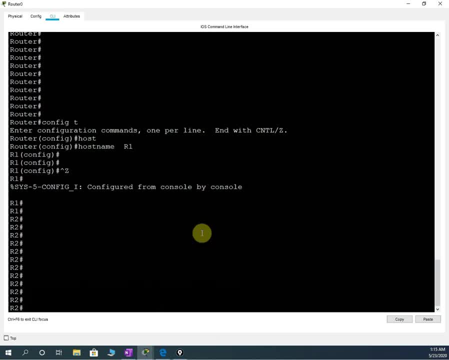 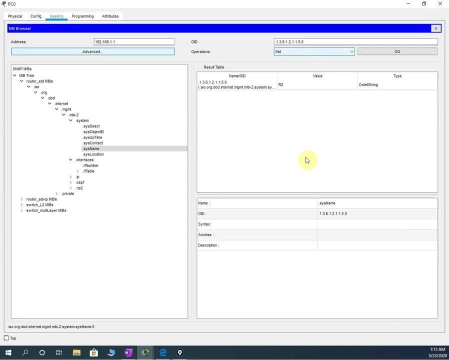 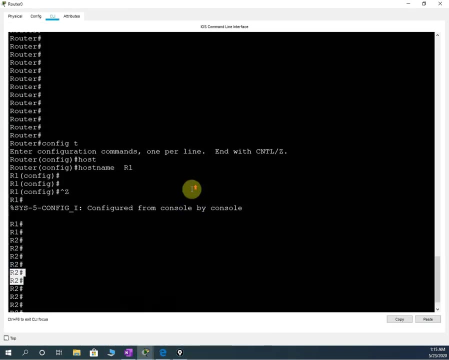 to R2. now we have R1, if you see. now it is changed to R2. so in this simple lab, what we are doing actually, in this lab, I am showing you how to configure the router, okay, how to configure the router with this protocol and in the packet tracer. we don't have all features in generally. 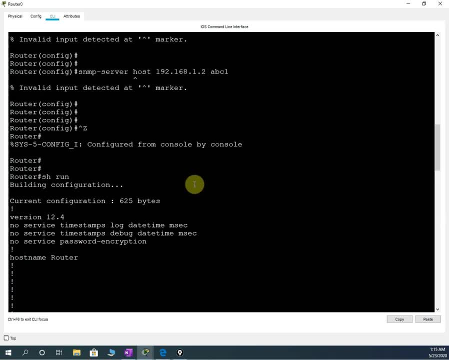 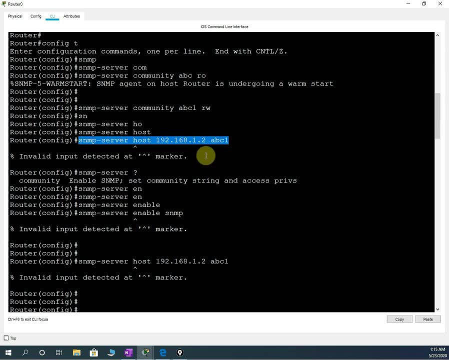 whenever we are doing the lab in gns3 or evng, we will type this command also, but this command is not taking the packet tracer. without taking this command, it is working in the packet tracer, but in real life, we are typing this one to execute this one. okay, what we need to do, let 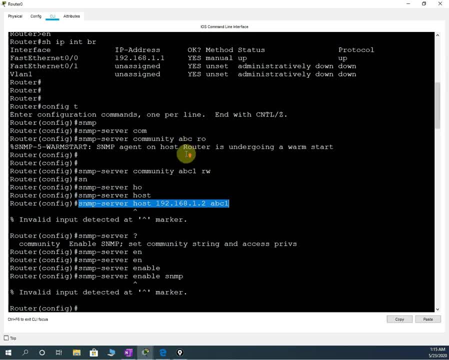 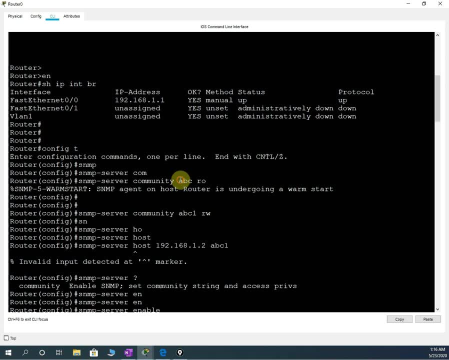 me revise this one. first of all, in the router, what you will do? you will go here in the router, you will write SNMP, server, community. then after that, this is assume a password, whatever password you want to give, you will write that password and you will write- arrow means read- only then. 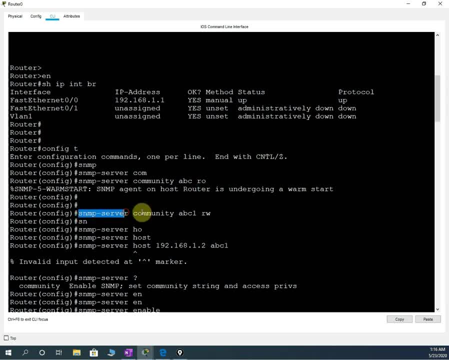 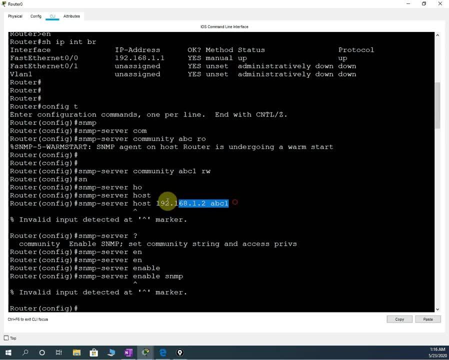 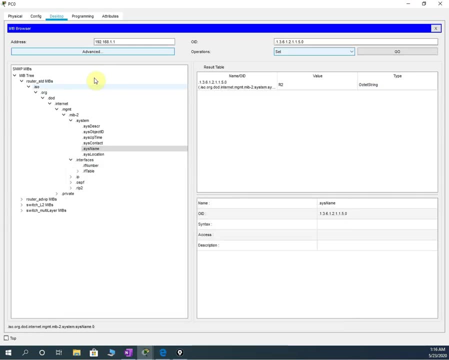 you will write SNMP, SNMP, server and community, then again the password for the right. okay, I wrote ABC one. then after that you need to assign the host. but it is not working in the packet tracer, so we will leave this one. and after that, after finishing this one, you will go in the 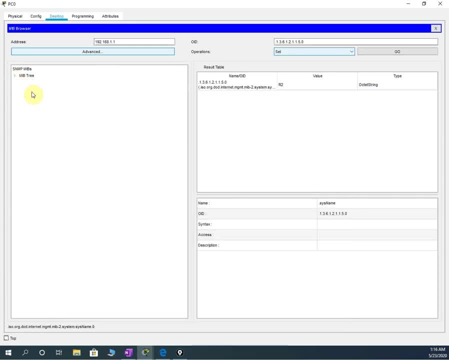 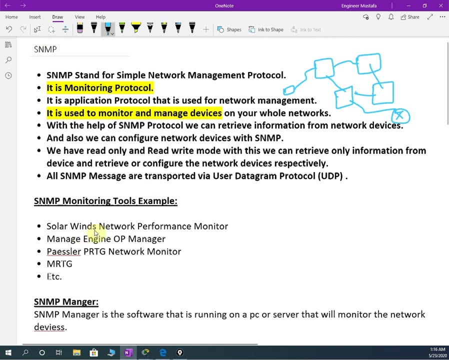 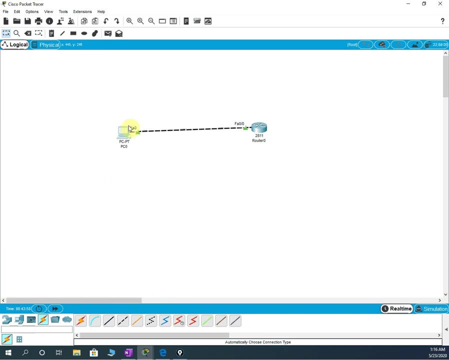 your supplier software, whatever software your company is using for the network management. we have many software, example I shown here: like we have solar wind, we have managed engine, we have MRTG, we have different. whatever software you have you will go there in the computer. this computer we are saying as a like network management computer, NMS, we are saying 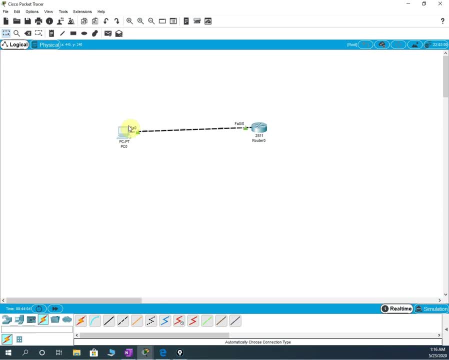 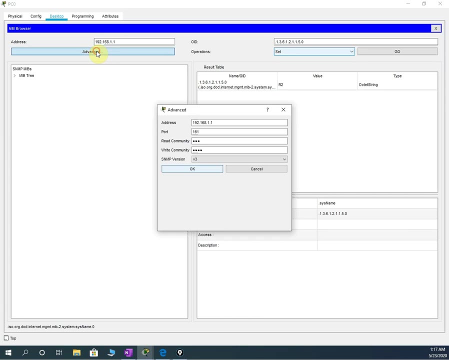 network management system or network management terminal NMT. we can say NMT in the network management terminal. we install that application and after doing the configuration, we will go here in this application and you will assign the IP address of the router and then you will press Advance and then you have here. you need to write the password, whatever you assign, for 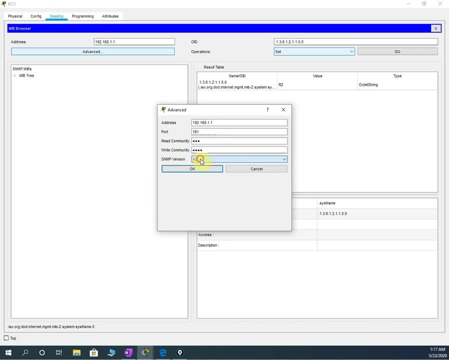 the read Community, right, Community, and you need to select which version you want to use and press okay. after that you will maximize this mib tree and in this one you will go inside and here you have the system detail. you will select the name if you want to see name. we have many feature here. 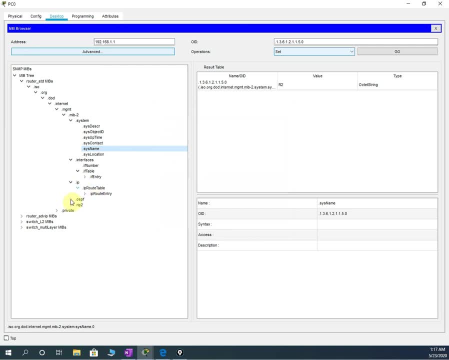 you can try. you will go here if you want to check routing protocol and rip or eigrp, whatever the advantage means. advanced features you want to see, you can see. but all features are not available in packet tracer but this one is available. you can try. I did not configure the packet tracer as we 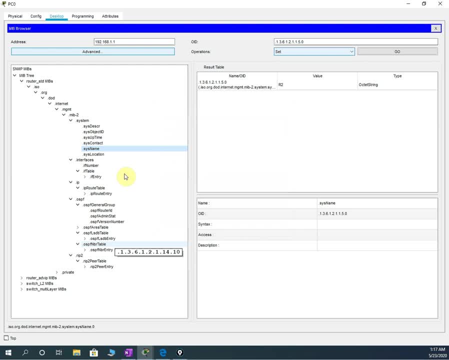 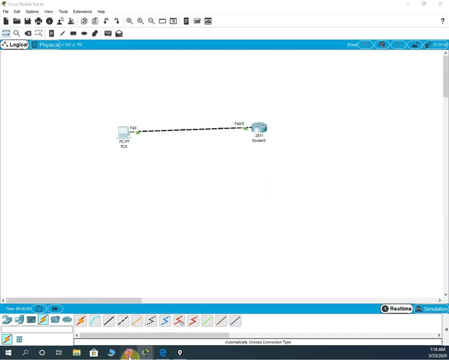 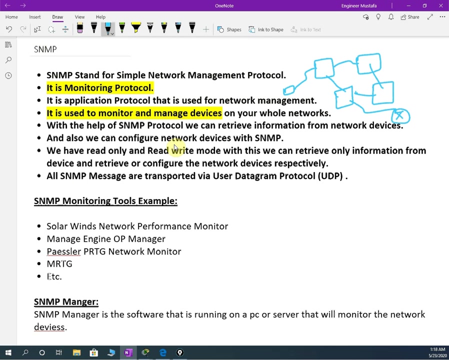 don't have in our syllabus the configuration only. we need to understand what is this one? okay, so that's why I given high level lab only. but before closing this video, let me revise. so see, imagine if you have a large network in your organization. you have many switches, routers and many servers. 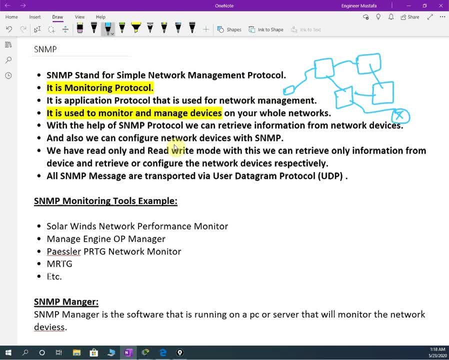 hundreds of workstation and it is difficult to monitor all like uh. if you have one or two devices you can easily monitor, but it is very difficult to monitor so many devices. so nms is a network management system. it is used to monitor a large number of network. 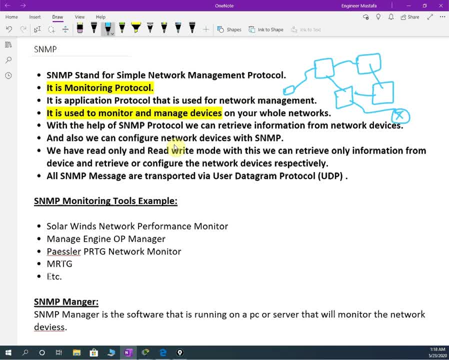 with this one, you will have the one PC. in that computer you are getting all the information. if you are integrated with the SMS system, you will get the message in your mobile saying that for this router you have this issue. like this: depending upon your company design and your organization, you can use like this: you will. 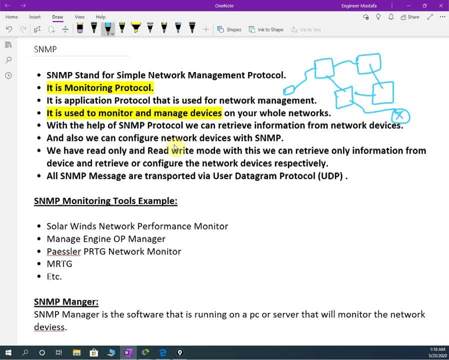 get when SMS in your router saying what is a problem, from which router? we have that feature also, but depending upon the organization, you will use that one, okay, so now, this is just remember. it is a monitoring protocol. it is used to monitor the network. if we have many devices, we cannot monitor. 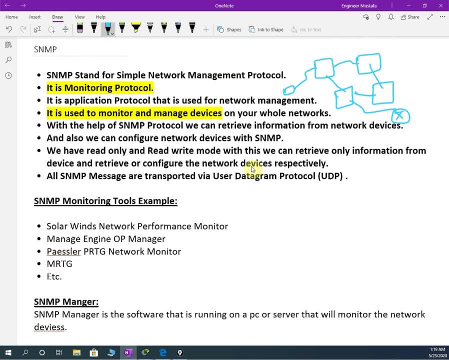 so it is easy to use one application and install in the one PC and the PC which we are. we install this application. it is, it is known as SNMP manager and the other devices which is going to send the data. that devices is known as agents and we configure agents and then agents is going to send the data to. 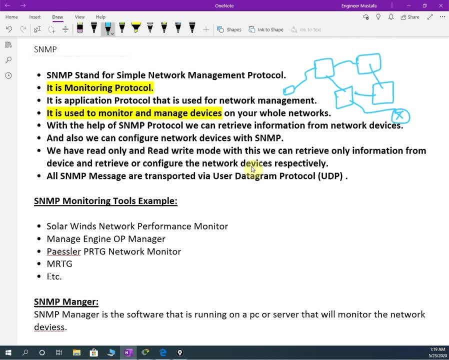 server and server is going to plot the graph and it will show us the utility of the CPU and how much internet we use, what is a bandwidth and which user use more bandwidth, which user use less bandwidth user. also, if we use more bandwidth, we can block for four hours, five hours like that we can do so. 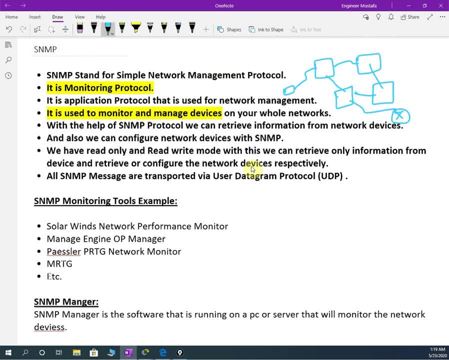 with the help of SNMP manager, we can read the configuration, read the parameter, as well as we can write, we can retrieve the information and we can configure the information also. okay, so this is a simple. only don't take like this is a big thing. this is a small protocol actually, whenever we want. 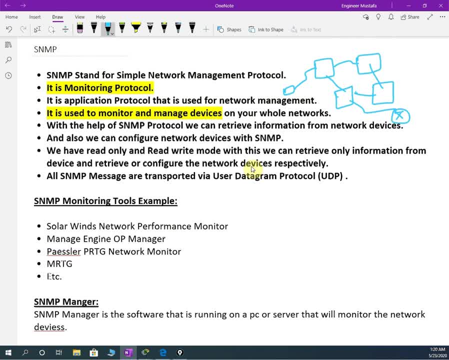 to do troubleshooting. we use many tool, like we will use ping, we will try to ping from one switch to another switch. it is working or not working. and we will use debug and conditional debug. actually debug we should not use in our production network. whenever we are, we are having the organization and it is working. don't use open. 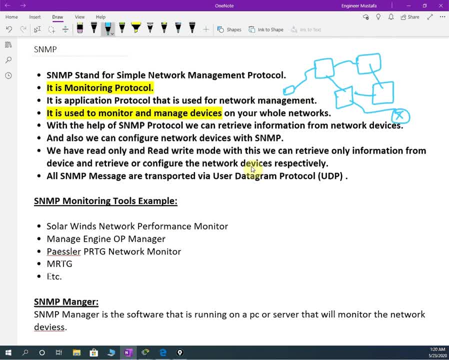 like we are going to open the debug in the router. so we are getting like for troubleshooting we are using, we are going to discuss that one in ccnp that is debug and unconditional debug. conditional debug and the unconditional debug- that is nothing but debug. we will open in the router so it will utilize more CPU and it will show us what is packet. 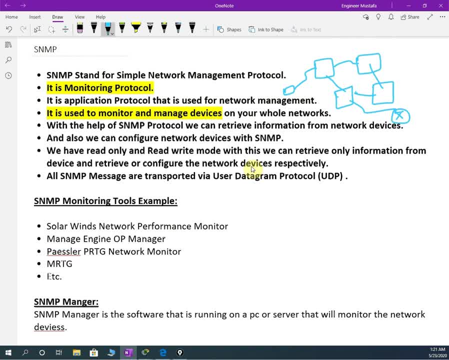 is going or not going, but it is not recommended to use in the production Network. if you don't have any option to do the troubleshooting, then only we use that one debug or unconditional debug. else we are going to use ping or trace route to check the issue or we are using the syslog. we have one more.